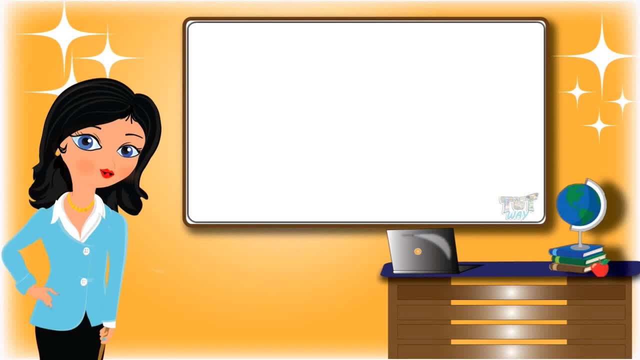 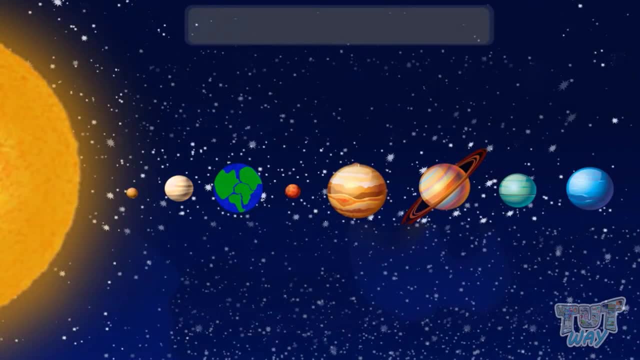 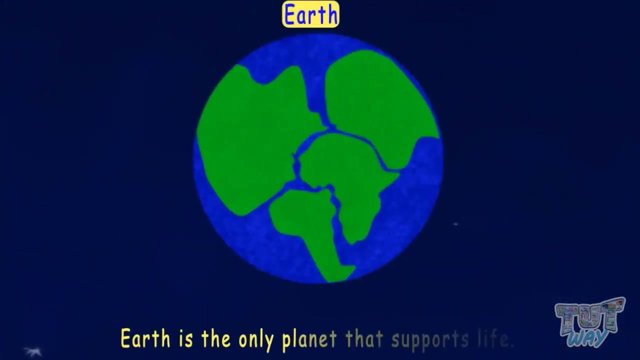 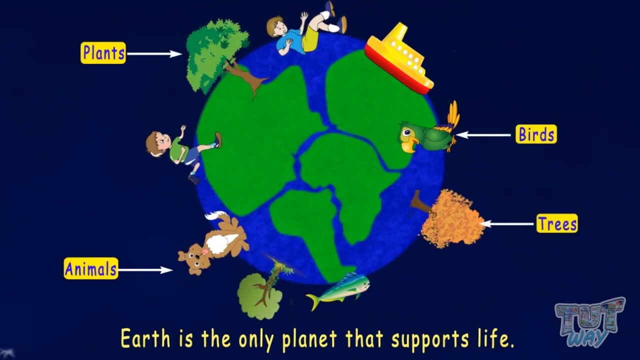 Hi, kids. Today we will learn about our planet Earth. So let's start, Kids. we all live on the same planet, which is called the Earth. Now let's learn some facts about our planet Earth. Earth is the only planet that supports life, as plants, animals, birds, trees, all human beings, all can live on this Earth. 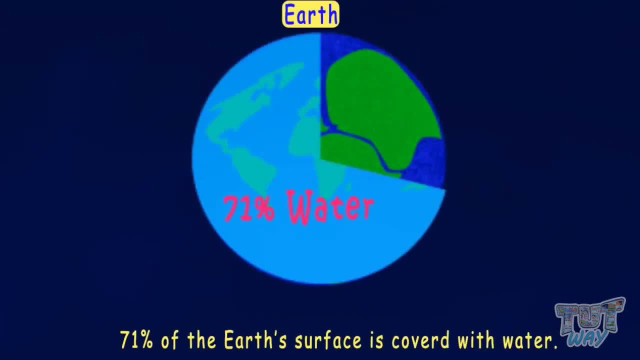 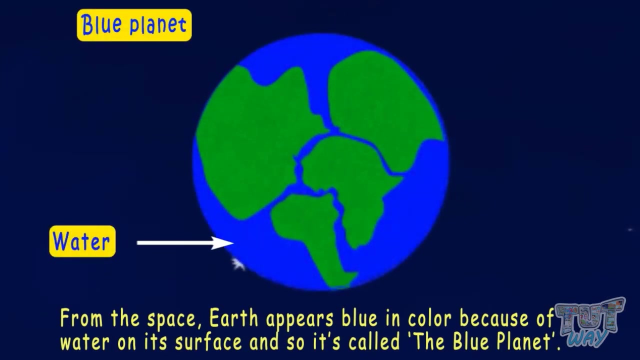 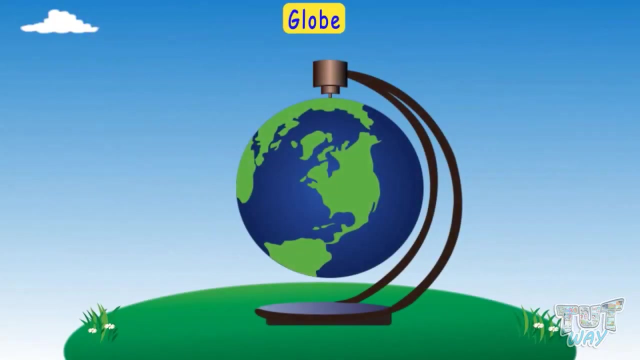 71% of the Earth's surface is covered with water. The rest is covered with land Land. From space, the Earth appears blue in color because of the water on its surface, and so it's called the blue planet Globe. Globe is a model of our planet Earth. 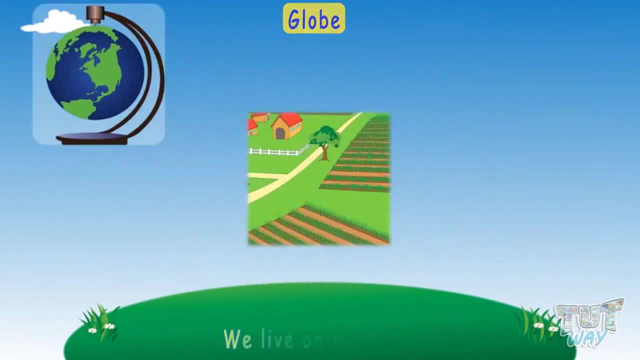 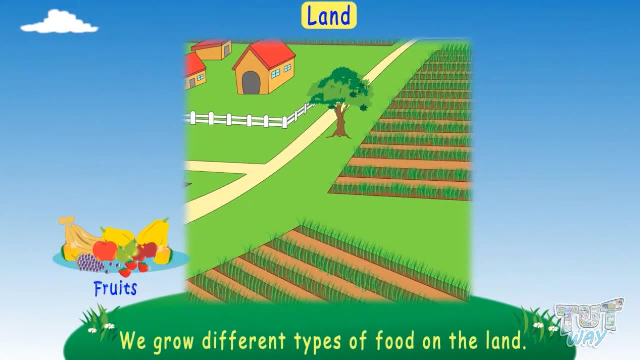 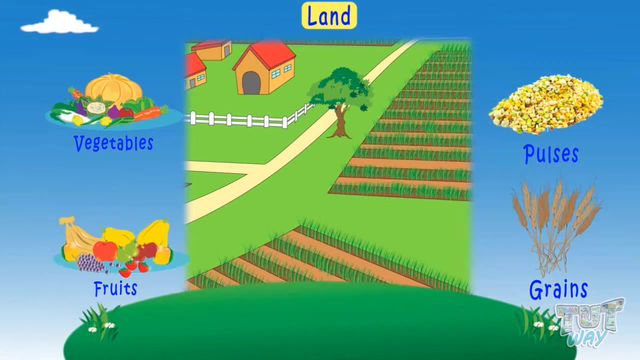 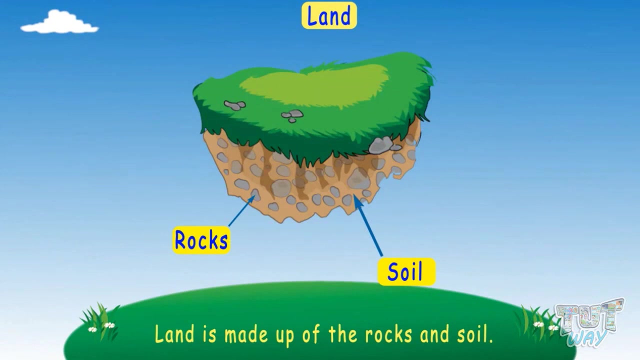 Earth is round in shape and we live on the land. We grow different types of food on the land, like fruits, Vegetables, pulses and grains. The land is made up of rocks and soil. Now let's see different landforms. 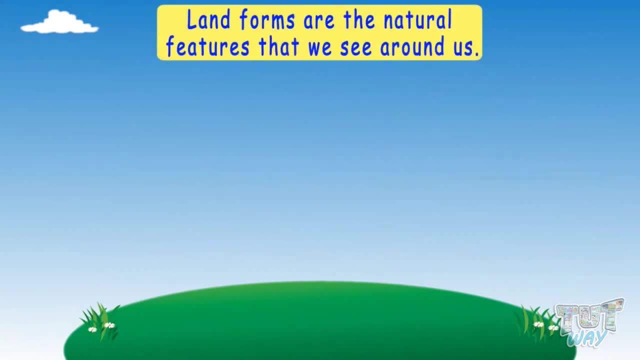 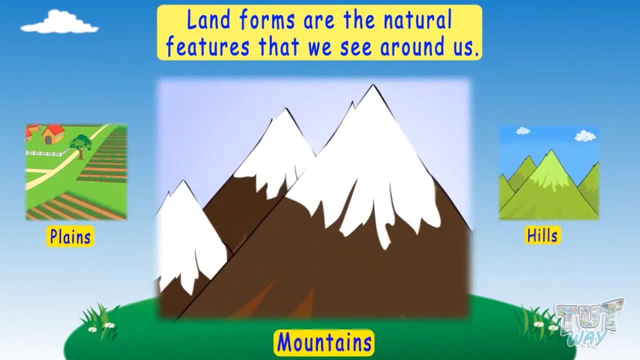 Landforms are the natural features that we see around us. Different landforms are planes, hills, mountains and rivers. Lands have their own FC Lands have their own E Lands have their own T Lands have their own T Lands are other fields, water bodies, deserts and valleys. 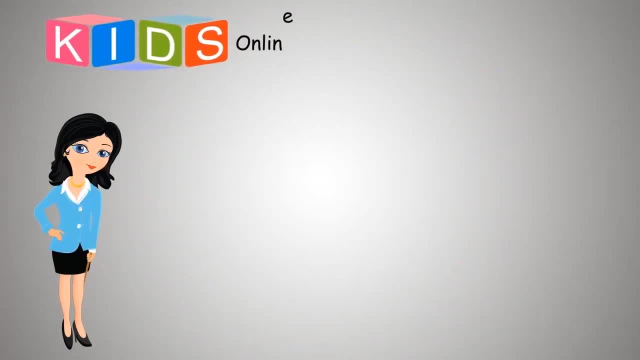 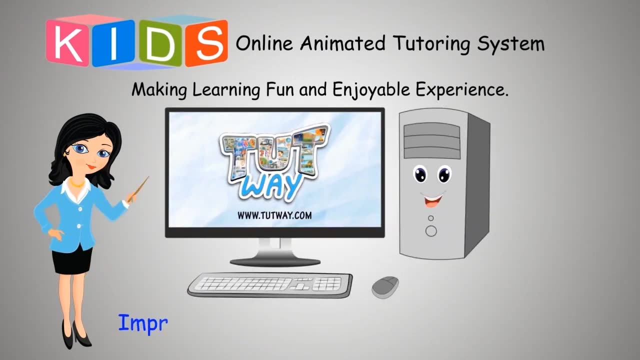 Now let's learn different types of landforms one by one. Laatwe has thousands of animated videos on Math, English and Science to clear the core basics of Planes. Tlw has thousands of animated videos on Math, English and Science to clear the core basics of Planes. 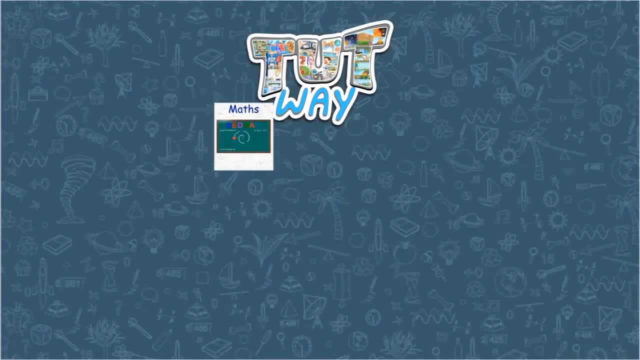 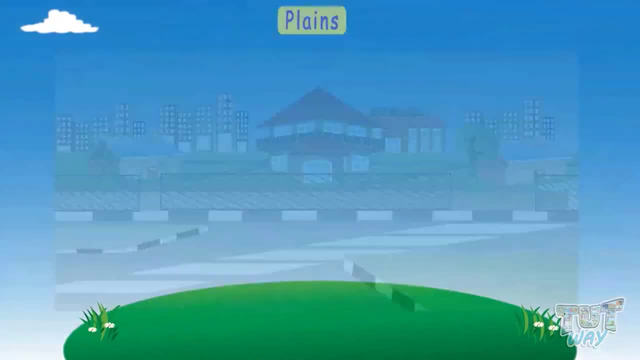 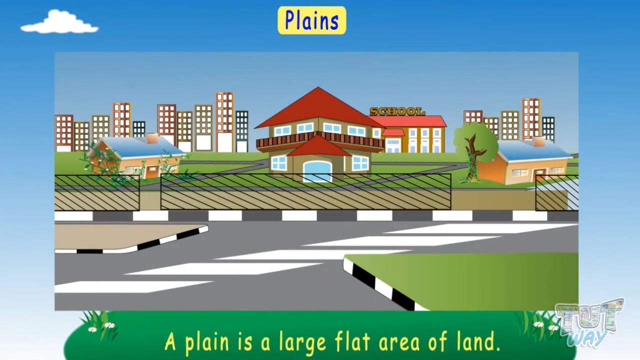 thousands of animated videos on math, English and science to clear the core basics of these subjects. Planes: A plane is a large flat area of land. Houses, buildings and roads can be easily built on planes. Hills: The land that is higher than. 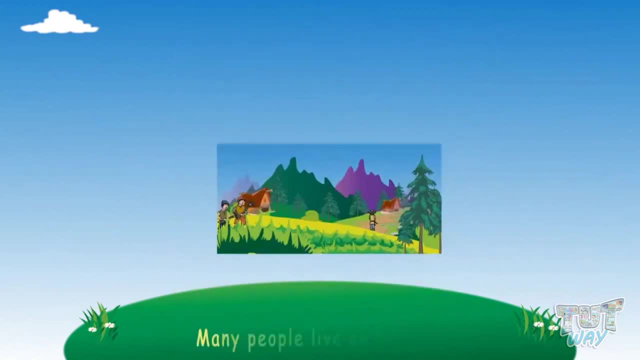 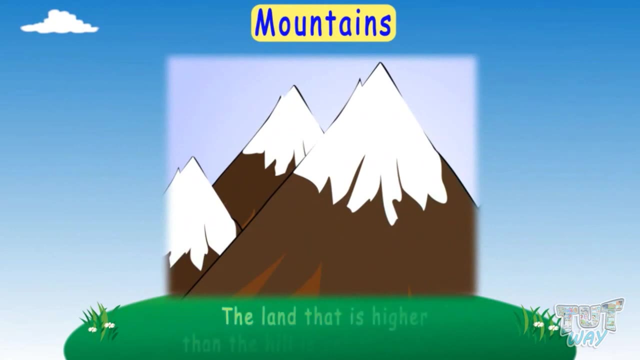 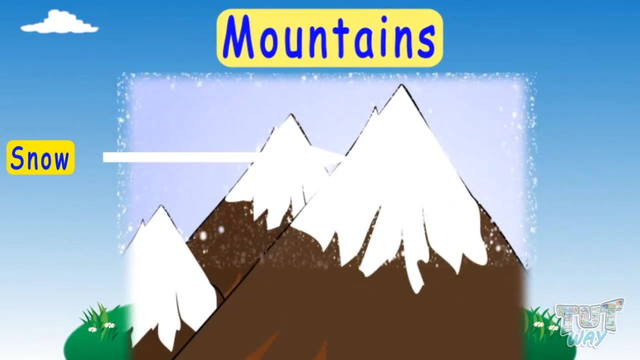 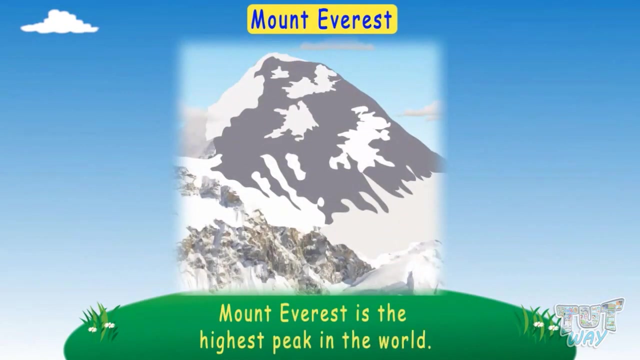 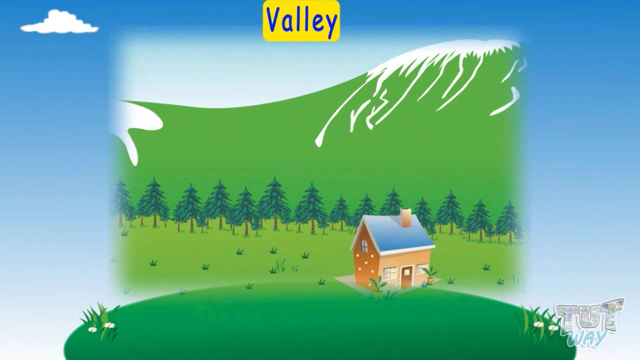 the plains forms hills. Many people live on hills, too. Mountains- The land that is higher than the hill- is called a mountain. peak Mountains are mostly covered with snow. Mountains- Mount Everest- Mount Everest is the highest peak in the world. Now let's see what is a valley. The low flat area between two mountains is called a valley. 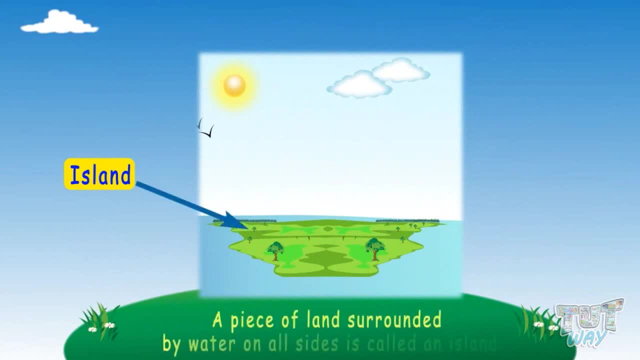 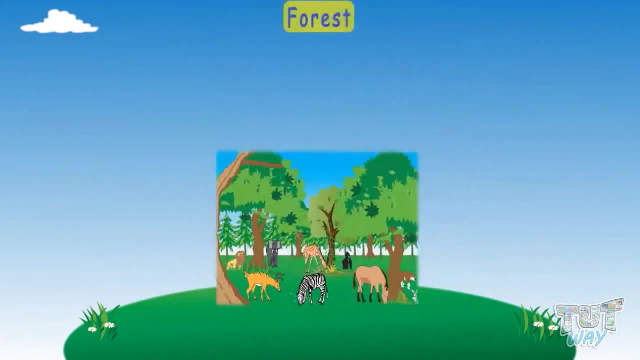 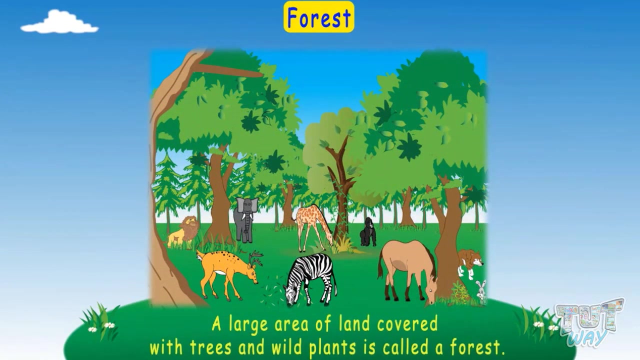 Island. A piece of land surrounded by water on all of its sides is called an island Mountain. A piece of land surrounded by water on all of its sides is called an island Forest. A large area of land covered with trees and wild plants is called a forest. 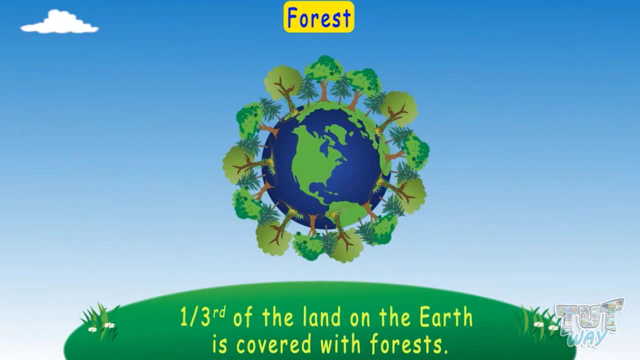 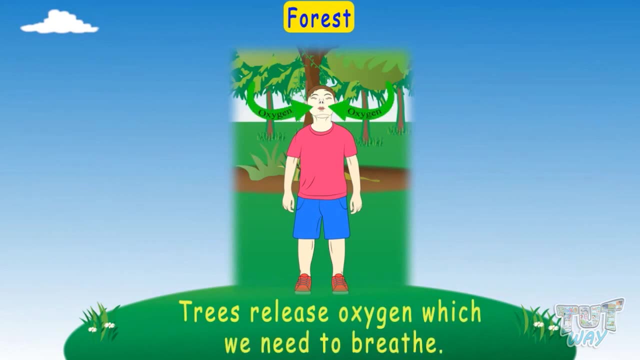 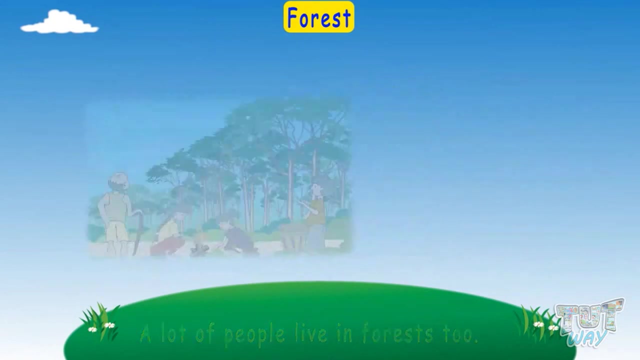 One third of the land on earth is covered with forests. Forests helps us breathe, As trees release oxygen, which we need to breathe. A lot of people live in forests too. Forests provides us with medicine and health care. Forests provide us with food and water. Forests provide us with 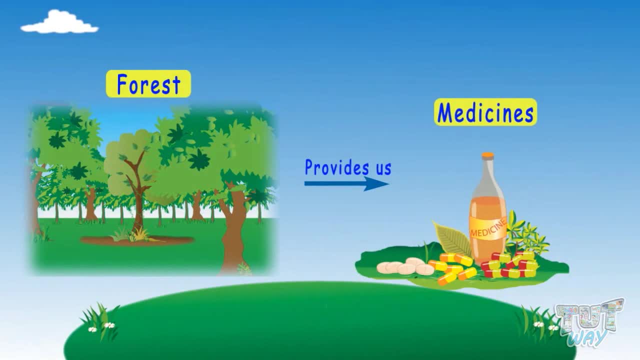 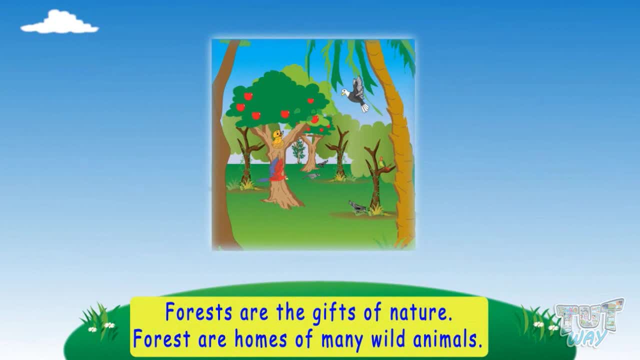 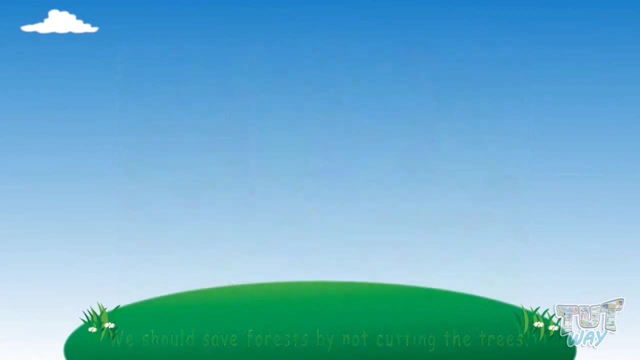 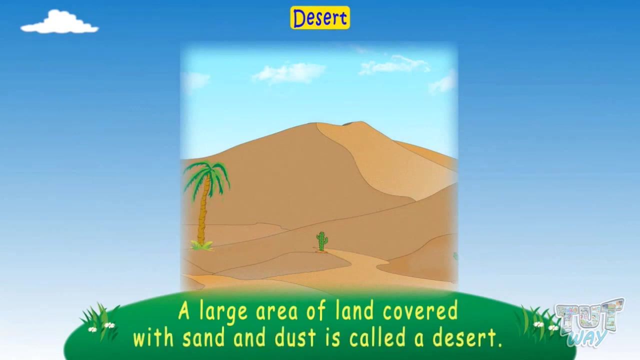 gifts of nature. Forests are homes of many wild animals. They provide shelter to wild birds and animals. We should save forests by not cutting the trees. Now let's see what is a desert. A large area of land covered with sand and dust is called a desert. Very few plants, such as cactus, grow. 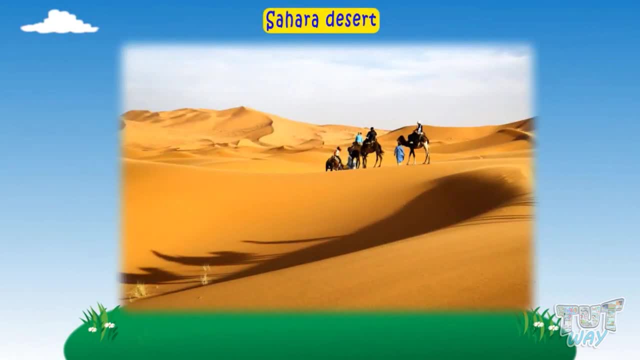 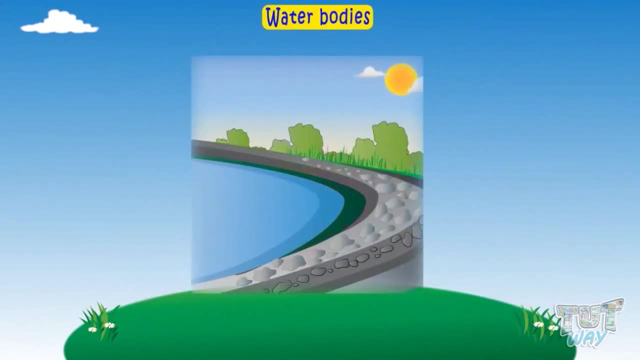 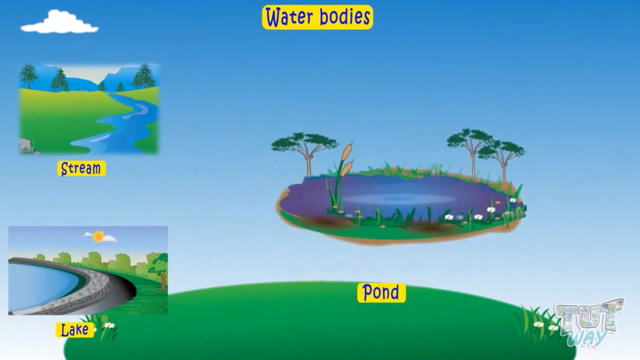 in a desert Sahara. The Sahara Desert is the most famous desert of Africa. Now let's learn about water bodies. These are places on earth where a lot of water gets collected. Such places are called water bodies: Streams, lakes, ponds, rivers, sees, oceans, different types of